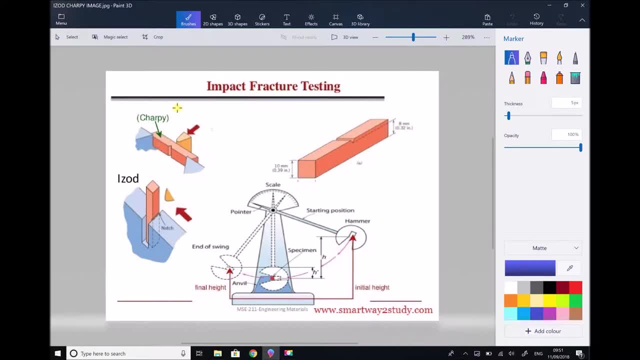 diagrams to show the differences. If, first of all, we look at the Sharpe test, what we notice is that the impact force is going to cause this to bend. It places a bending stress on the piece of material And what we have is we have a notch cut in the centre. 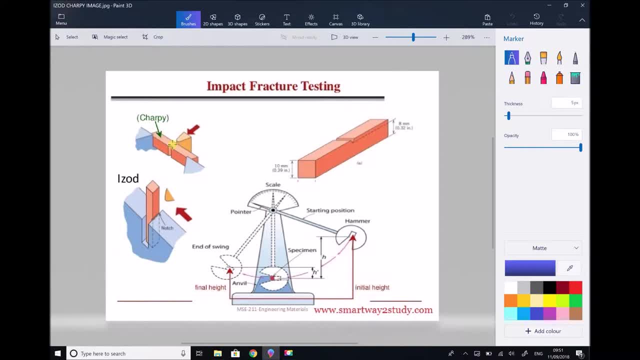 to enable the piece of material to fracture at a specific point. What we're interested in in the Sharpe test is the area, or the cross-sectional area at the notch, because that's the point where the material is going to fail, Providing we use samples of the same. 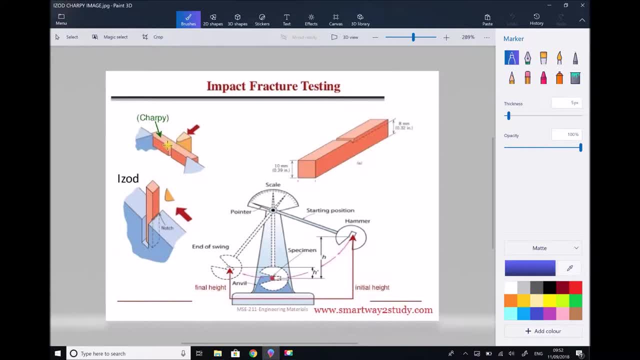 size and same cross-section, then we're able to get the same cross-section of the material. Now what we notice is that the impact force is going to cause this to bend. It places a comparison of how different materials perform under impact. Now the Izod test is slightly. 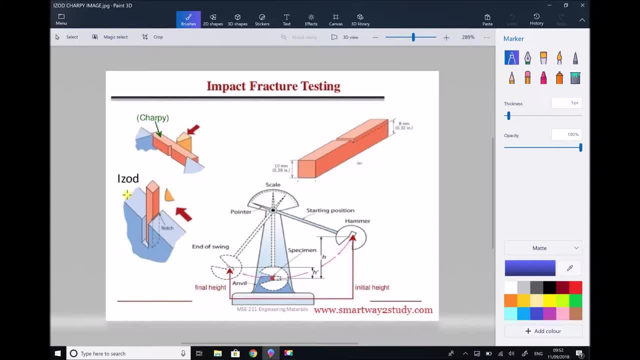 different, And instead what we have is a kind of shearing action. Once again, we have a notch cut in the material, And the reason for that is to ensure that the material is going to fail at the correct place, And once again we would have calculated the area at. 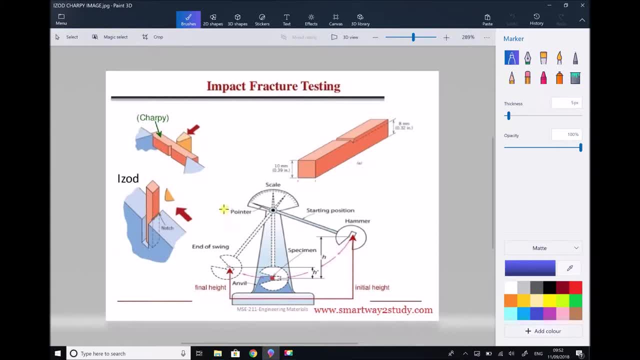 the notch, the cross-sectional area, And with the Izod test, what we end up with is a shearing action. So let's focus on the Izod test Now. what we see at the bottom here is an example of the machine that's used: the Izod. 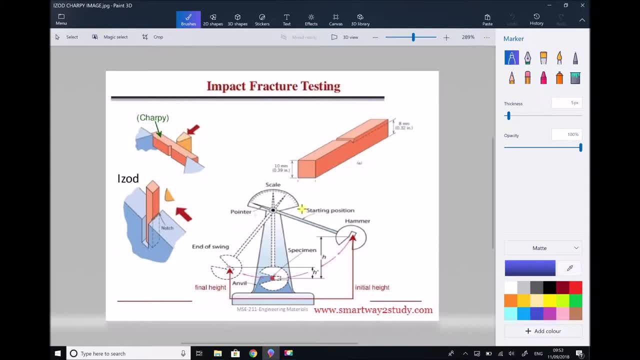 tester. Now what happens here is we lift the hammer on the right-hand side And in doing so, we give it potential energy. When we release that hammer, it's going to swing and it's going to strike our test piece, which is going to be positioned in the center here. 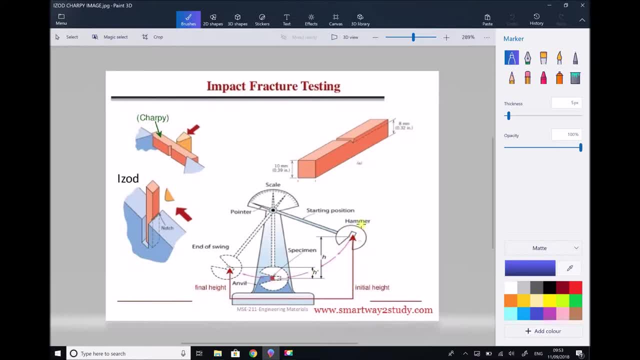 Providing we give the hammer enough energy by lifting it high enough and using a heavy enough hammer, then that piece of material is going to fail And, as it fails, it's going to absorb some impact energy. Now what that means is that the hammer isn't going to swing as high as it was released from, because some of that 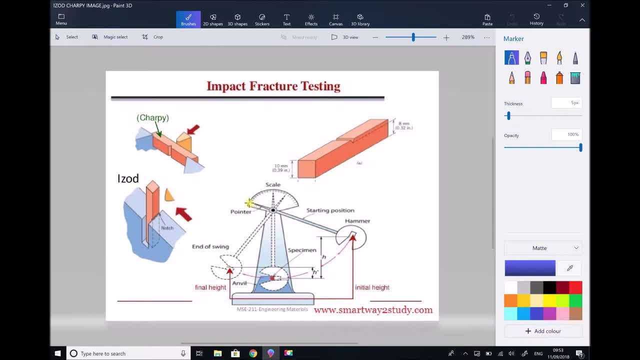 energy is going to be lost, And what we end up with is two readings. We end up with a starting reading and a finishing reading, And from that we're able to calculate the amount of energy absorbed by the test piece And, as you would expect, different materials. 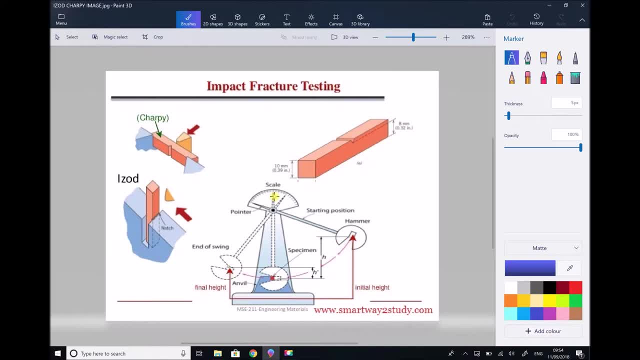 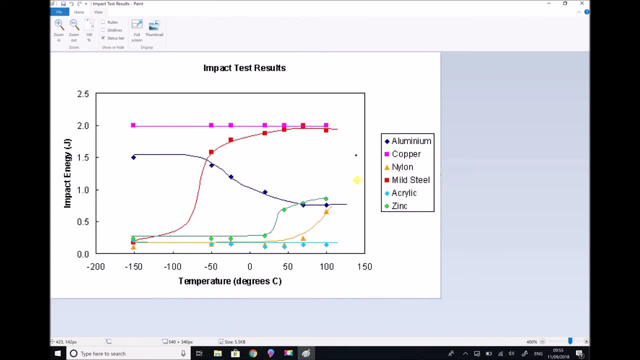 will be capable of absorbing different amounts of energy. Let's take a look at some typical results from this type of test. So here we have some results that have been generated from an impact test, And the first thing that we notice is that a number of different materials have been tested: Aluminium, copper. 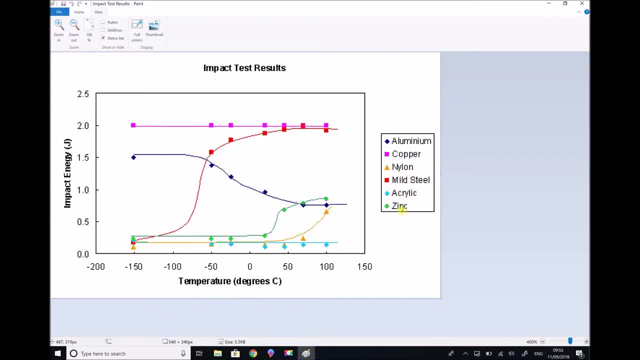 nylon, mild steel, acrylic and zinc. Now on the y-axis, on the left-hand scale, we have the amount of impact energy absorbed. Now, what this isn't factoring in is the cross-section of the material. So in actual fact, this should be impact energy per unit area, And that would be dependent 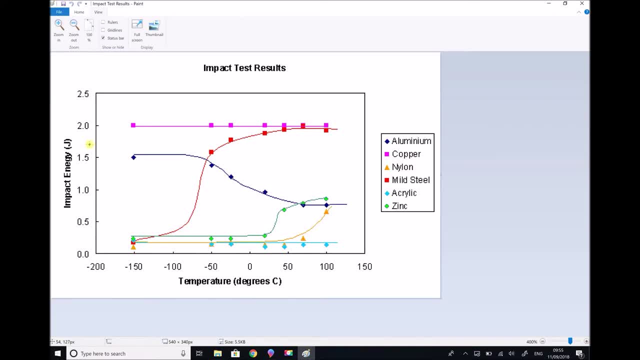 on the cross-section of our material, but at least it gives us a representation of what happens in the test. From this we can immediately see that our toughest material is copper, because it's able to absorb the most impact energy. But the other thing that we notice is that there's 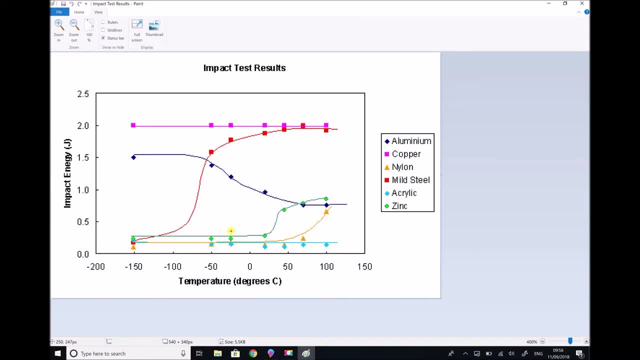 variations throughout different materials, And the variations are variations with respect to temperature 0 scale. here we have temperatures ranging from minus 150 degrees C all the way up to 100 degrees C. Now, what we notice is that between those ranges, the toughness of copper is unaffected, But let's take mild steel as an example. What we notice 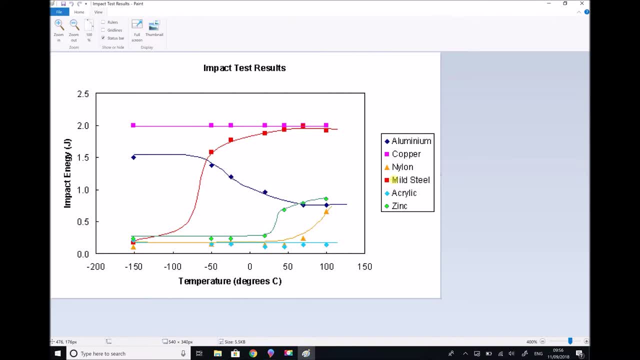 with mild steel is the toughness varies dramatically with temperature. So at low temperatures, here we see the amount of energy absorbed being very low, but between minus 100 degrees and minus 50 degrees we see a huge increase in the toughness of our steel. What that demonstrates is that at low temperatures, 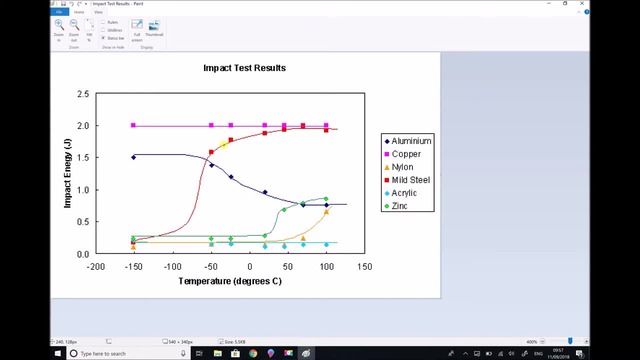 steel loses a lot of its toughness, particularly mild steel, And then, for temperatures above zero degrees, we see it having a comparable toughness to copper. Now aluminium appears to work the opposite. At lower temperatures, aluminium is tougher so at minus 150 to minus 50 degrees C, aluminium 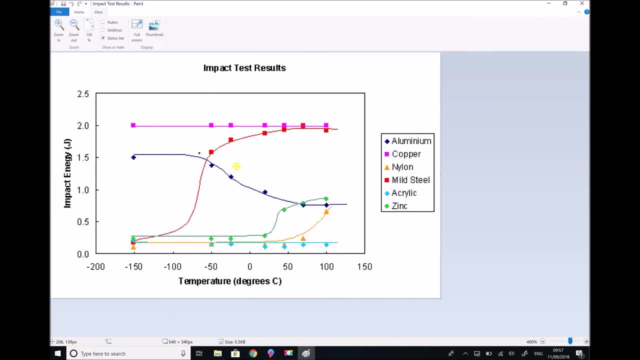 is not as tough. At lower temperatures aluminium is tougher. so at minus 150 to minus 50 degrees C, aluminium is not as tough, has its highest toughness, but by the time we reach 50 and 100 degrees C it appears to have. 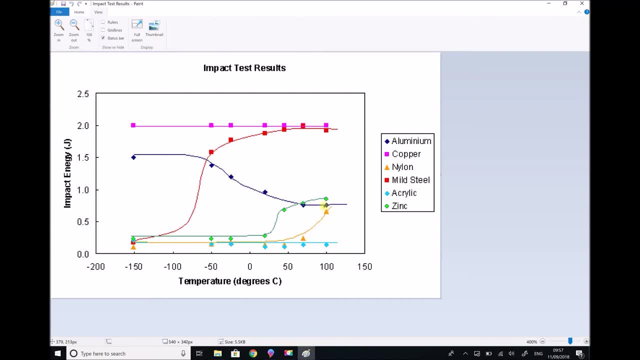 lost some of that toughness. It's less able to absorb impact at higher temperatures, And we also see variations in our other materials, zinc and nylon increasing in toughness at higher temperatures and acrylic remaining fairly constant, with the lowest toughness of each of those materials. So the important things to take from this video is, first of all, how the test is.